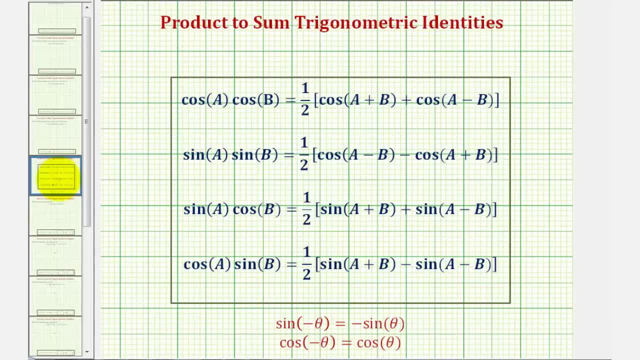 For a quick review, here are the product to sum trig identities. We'll be using these first two where we have cosine a times cosine b and sine a times sine b. There is one thing I do want to mention here, though. It's best to have the larger angle first, because it's better form to have a plus b and a minus b positive. 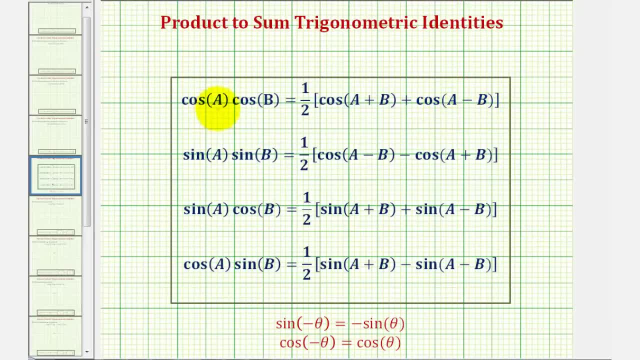 In order for a minus b to be positive, a would have to be greater than b. It wouldn't be wrong if we switch these angles, But if we had a negative angle for a cosine of a minus b here or here, it is better form to perform a substitution using a negative angle identity given here. 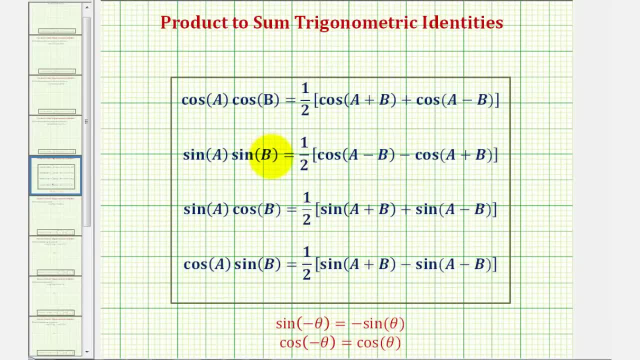 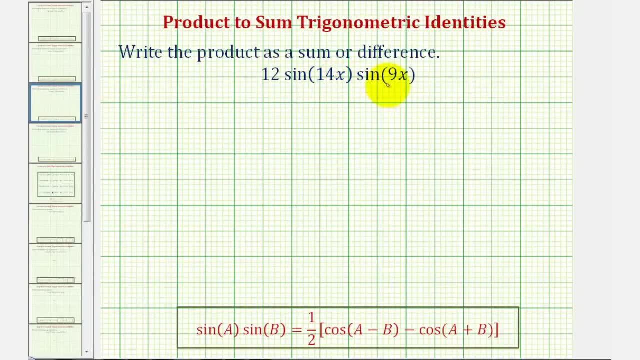 But again, we can avoid this as long as a is greater than b. So, looking at our first example, notice how, if x was positive, 14x would be greater than 9x. So we do have this in the preferred form, where a would be equal to 14x and b would be equal to 9x. 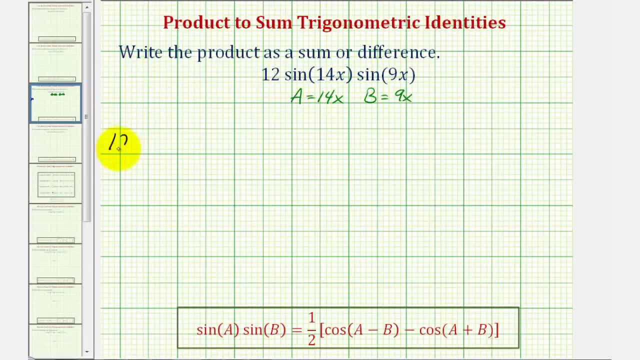 So, applying our identity, we can say that 12 times sine, 14x times sine 9x is equal to: we solve the 12 and then times one half times the quantity cosine a minus b. Well, a minus b would be 14x minus 9x, that's 5x. 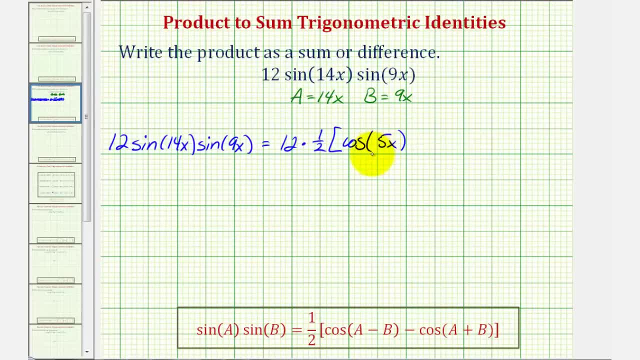 Notice how we do have a positive coefficient, which is what we prefer. if we have an expression, Then we have minus cosine of a plus b, or 14x plus 9x, which is 23x. Now we just need to simplify 12 times one half, of course, is 6.. 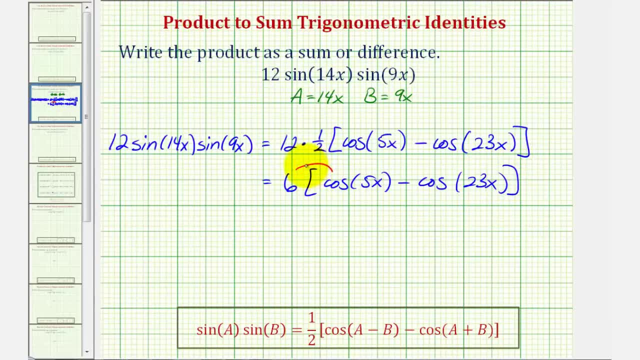 And we still have a product here. so now we'll distribute. So we have 6 cosine 5x minus 6 cosine 23x. Now we have the given product as a difference. Let's take a look at our second example.